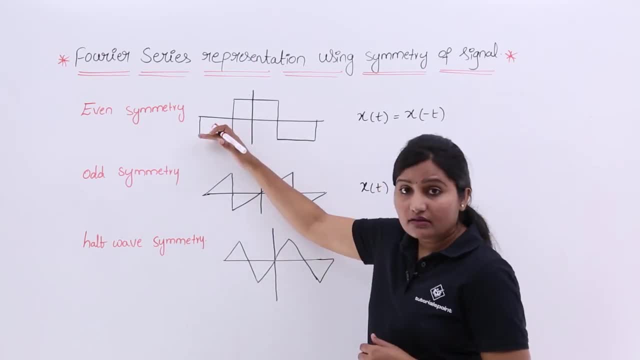 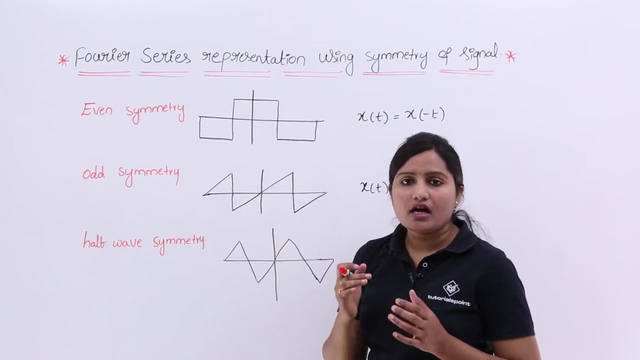 you are also satisfying half wave symmetry and you are having all odd harmonic cos terms. you are having That means cos omega naught t, cos 3, omega naught t, cos 4, omega naught t terms will be presented in the Fourier series representation. That means you are limiting. 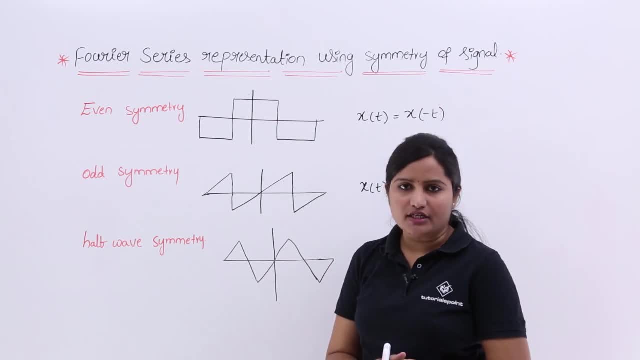 the representation terms in Fourier series representation. So here, if any signal satisfying odd symmetry and half wave symmetry, then In your Fourier series representation you are having only sine terms, that is also odd harmonic sine terms. So half wave if any signal satisfying half wave symmetry means 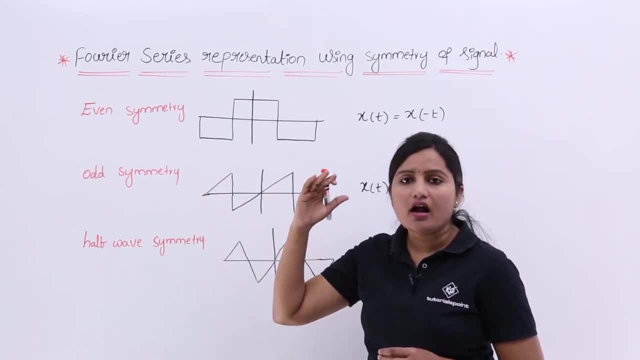 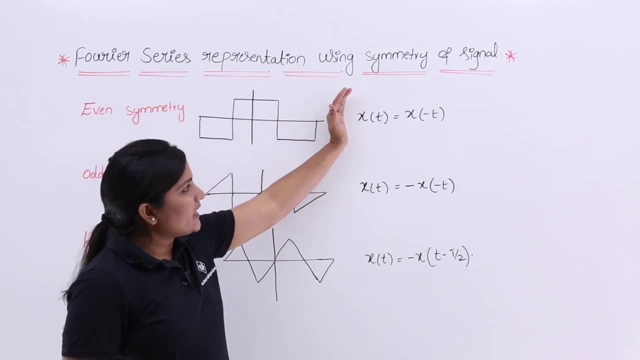 So definitely, whatever the harmonics are there, all odd harmonics are going to present. So now you can see the equations. So if x of t is equivalent to x of minus t in a half wave period, Then If the signal is satisfying in this condition, then the signal is said to be even symmetric. 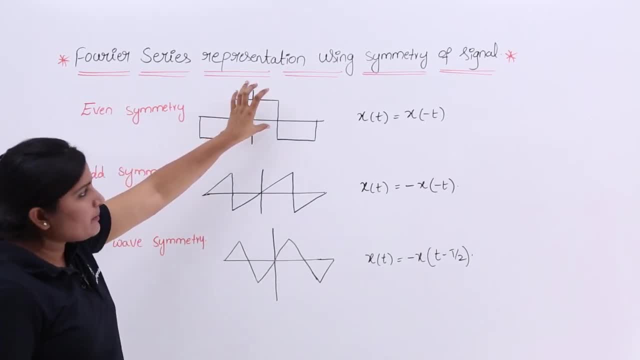 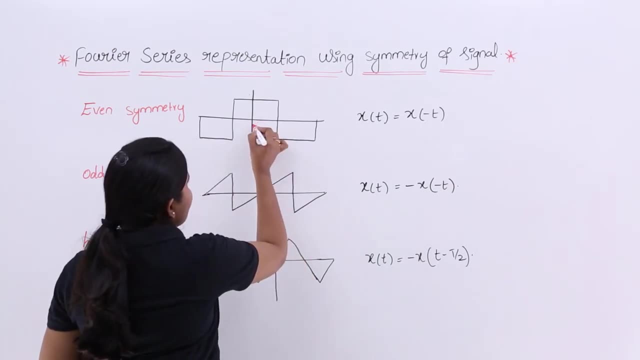 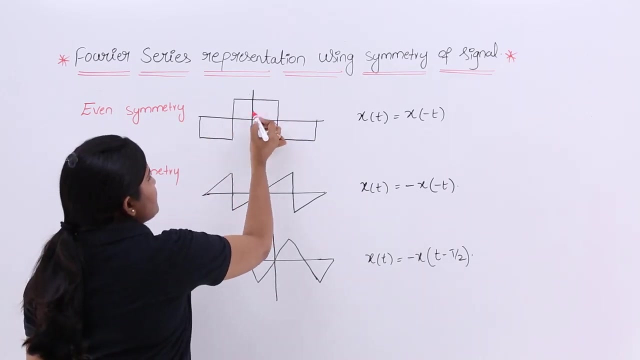 signal, For example, I am considering this signal, I am considering half duration of this signal. So here I am considering this half period duration. from here to here I am considering like x of t, If you consider x of minus t, So for this, the x of minus t. 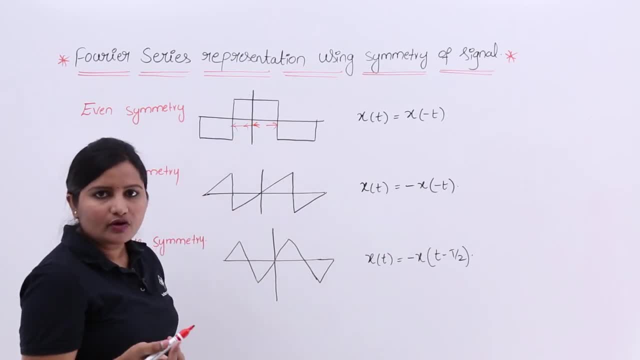 is this: These two are same. If you consider x of t, Then Then. and X of minus t, those two are said to be same. Coming to here, coming to odd symmetry, X of t is equivalent to minus X of minus t. So that means, if you are having X of t, that 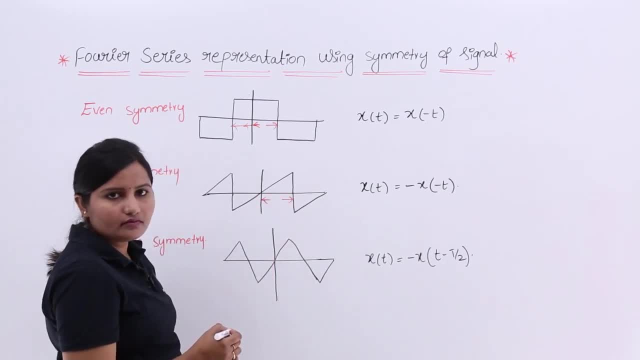 means I am considering this as X of t. The X of minus t for this X of t is reverse of mirror image of that. So just we need to fold the signal. this is X of minus t for this X of t. if this is X of t, this is X of minus t. If you want minus X of minus t, then it. 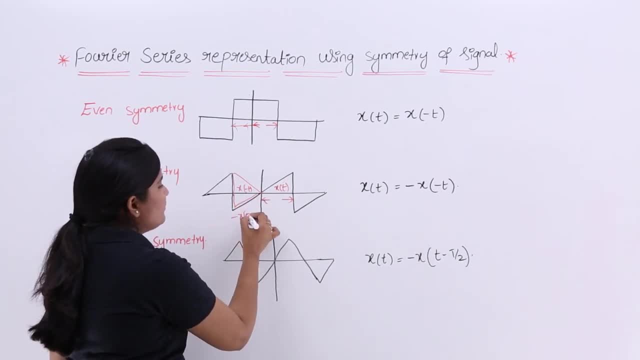 will reverse like this: So this is minus X of minus t. So now you can see if you consider this as X of t, if you consider a half wave period in a signal, and if you consider minus X of minus t, then this is X of minus t. So this is X of minus t. So if you consider 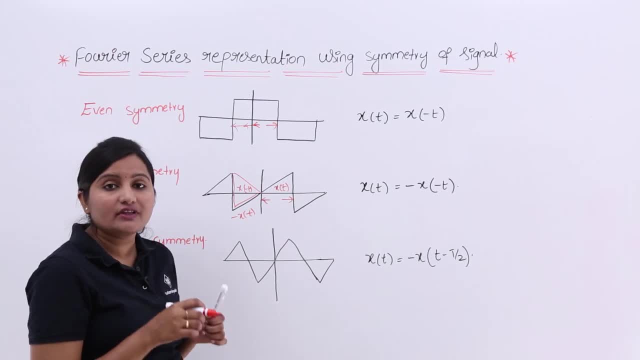 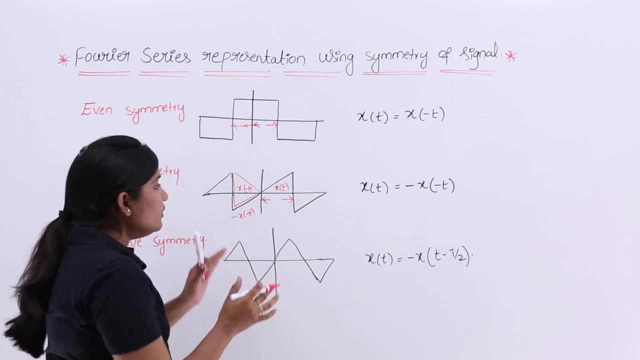 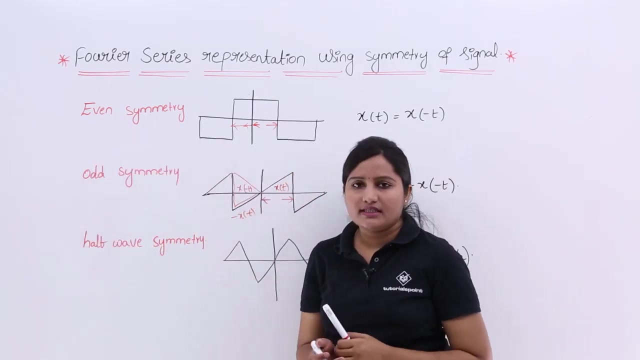 x of minus t for that signal it need to synchronize with the signal. So you can see it is equal to the actual signal processing. So now we can say if this signal is satisfying this condition. we can say: this is a odd symmetric signal which is having all cos terms, ah all. 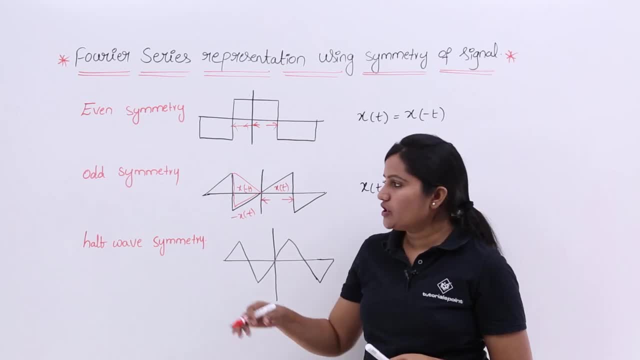 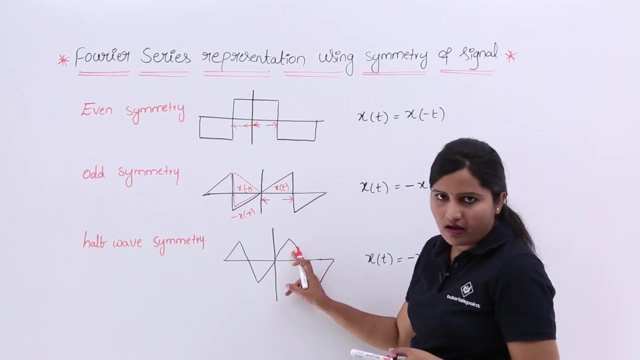 sin terms. So in Fourier series representation this odd symmetric signal is having only cos terms. Now coming to half wave symmetry. So here to satisfy half wave symmetry, for example, if you consider any half wave duration of the signal after shifting to next half wave position and reverting, you need to synchronize. 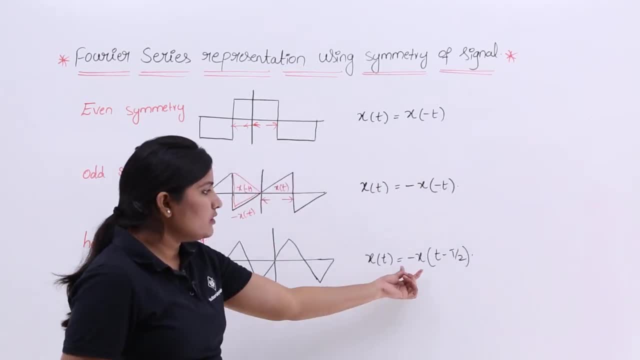 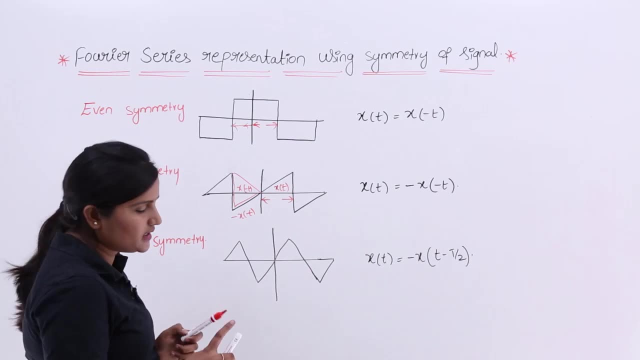 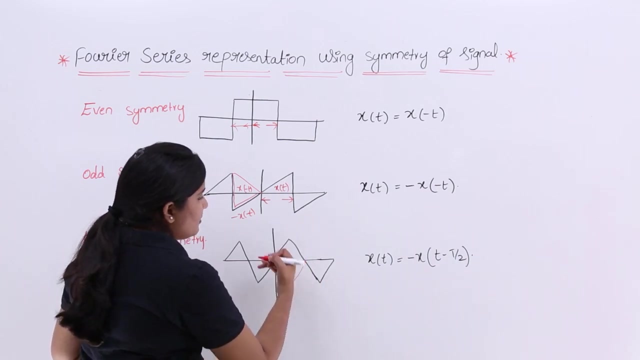 with the signal. So here, if you see. so if I shifted and reverted, that should be equal to your signal process, normal signal processing. So here you can see that this is the signal processing. So here you can see, I am considering this one, I am shifting this one to here and 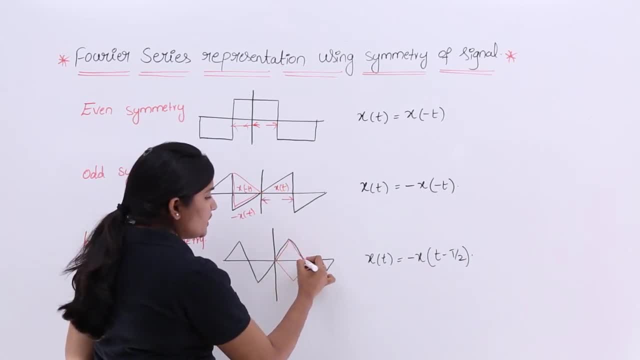 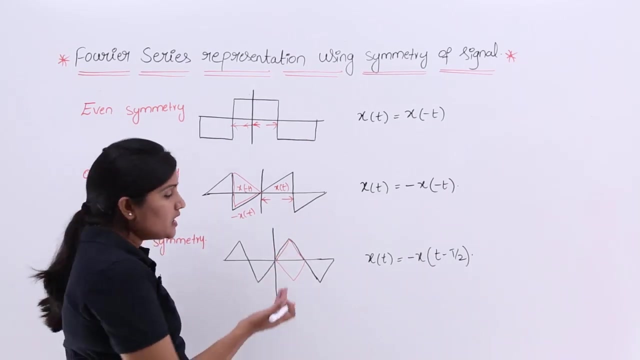 I am reverting. I am reverting means. So you are getting normal signal, processing this, synchronizing with the normal signal. So this signal will satisfy half wave symmetry and the same way this signal will satisfy odd symmetry also why? because, if you consider, 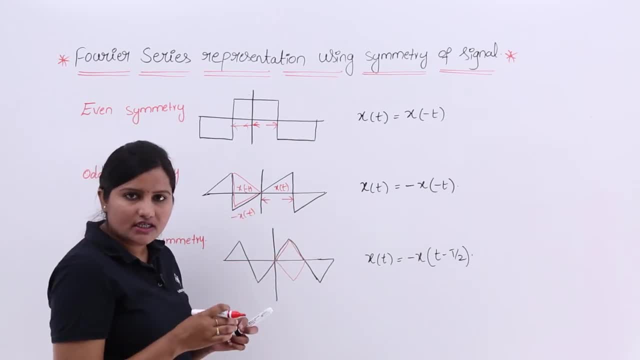 mirror image and reverted, you are going to get just Wide synchronous Odd same signal. that means odd symmetry. only you can confuse all odd symmetric signals. are half wave symmetric signals? no, not at all. all harmonic signals, not at all this half wave symmetric signals. why? because if you consider this signal itself, 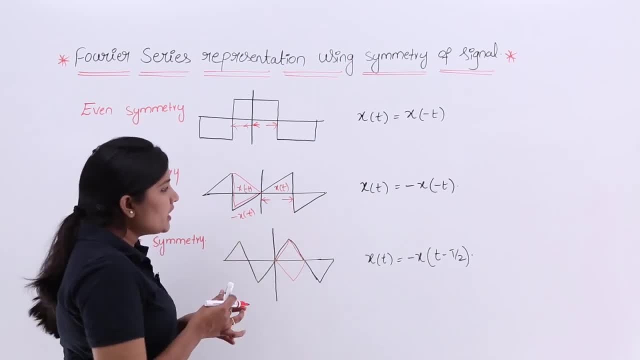 If you are shifting this position to here, that means like this, and diverting, reverting means you are going to that, like this. you are getting this signal. So now, Buddy, A common error, That means half waveשלing. 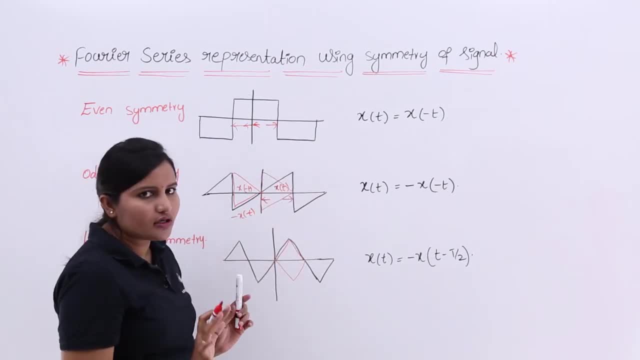 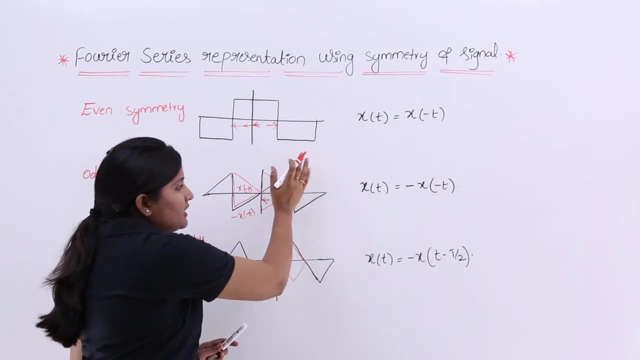 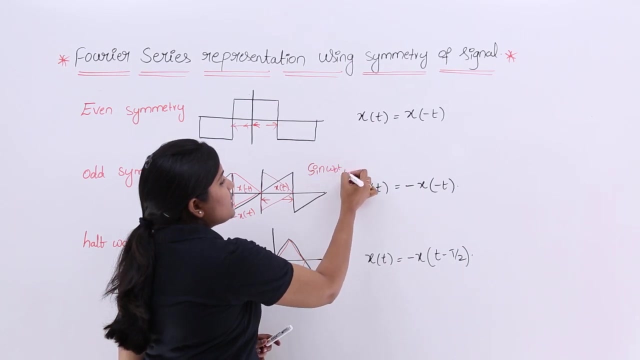 All Reality. So compared, No, you are not getting this signal. but this is odd symmetric signal but not half wave symmetric signal. In this signal all cos terms are going, all sine terms are going to present. then that means sine omega naught t, sine 2 omega naught t, sine 3 omega naught t, so on, are going to present. 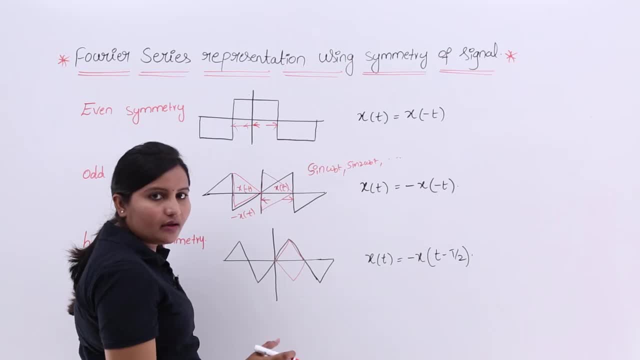 Now coming to this signal, this is satisfying both odd symmetry and half wave symmetry. So here both odd symmetry. half wave symmetry means here, if you consider this signal, then you are getting, so now. so this is odd symmetry. why? because if you reverted and shifted not shifted, if you consider x half minus t and you reversed in negative y axis, you are getting. 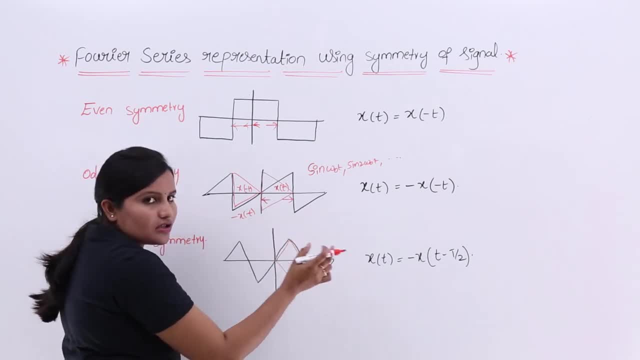 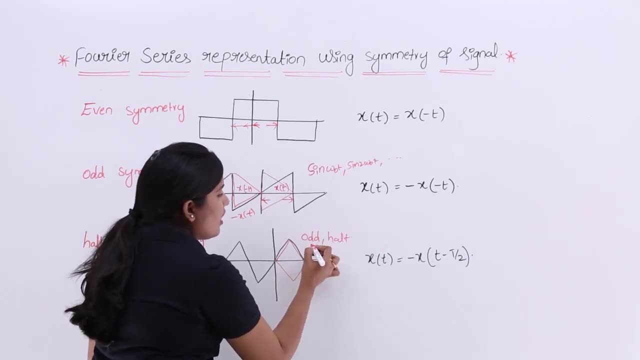 the same signal. or if you shifted and reversed also You are getting the same signal. So it is satisfying both odd and half wave symmetry. So odd symmetry means so you are having all sine terms. but as it is satisfying half wave symmetry also, so you are having odd harmonics, of odd symmetry, That means odd harmonics means sine. 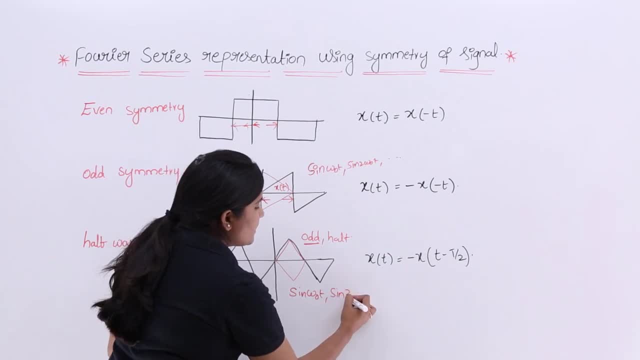 omega naught t sine 3. omega naught t sine 5. omega naught t will be present in the half wave symmetry. Later it will be transported back when there is no significant difference. So this is what you are having. So coming to r, Billy Fourier series representation. coming to here, this will 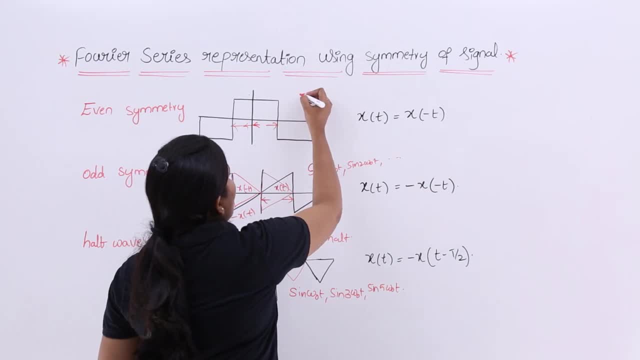 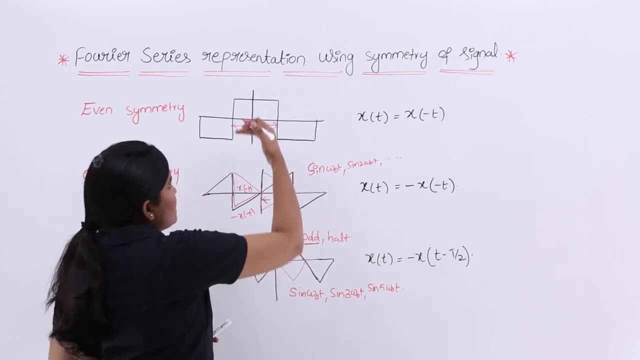 covers all cos and it will. satisfies this. symmetry or not, half wave symmetry or not means here you just shift and reverse. So if you shifted this to here and if you reverted to here, so this is having시고, So this is a little bit faster, So you yourself can shift and reverse here. So if you shifted to here and if you reverse, then you are getting same signal. so this is also satisfying both. even and even. So you also have enough«£»«»»»«££££«££££££££€«. Ireland is at liberation limit. 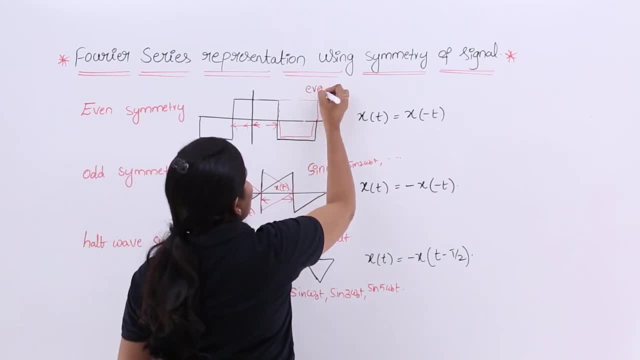 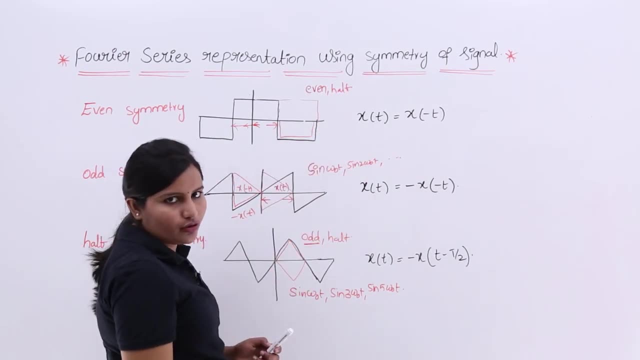 Then the neighbor is there in the right. Now let us call that ПотомắtgCh u Turertasetti. So this also satisfying, both even and half wave symmetry. So that is why, as it is satisfying even symmetry, cos terms are going to present. So in that cos terms also, as it is satisfying. 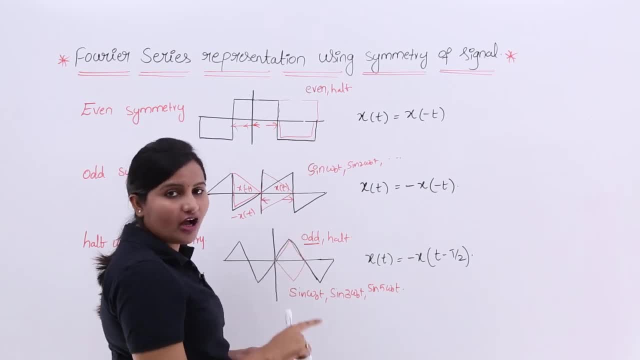 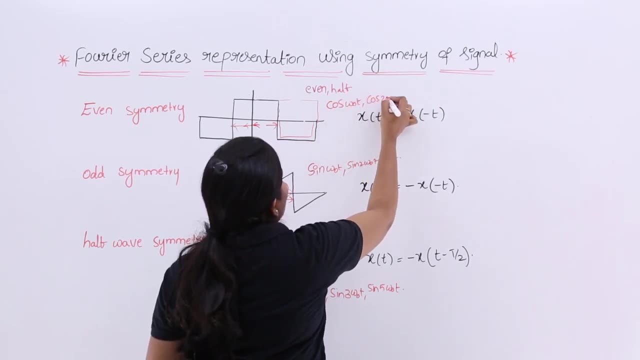 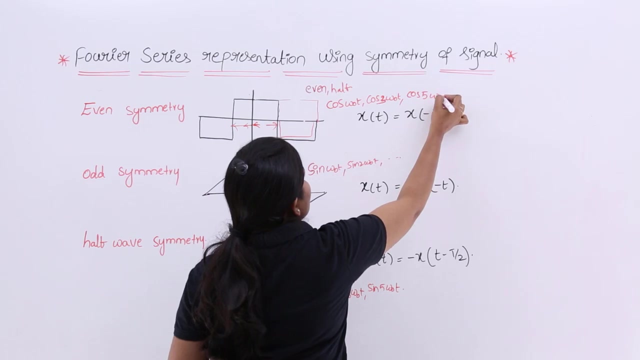 half wave symmetry, only odd harmonics of cos terms are going to present. Odd harmonics means so cos: omega naught t, cos 2, omega naught t. odd harmonics cos 3, omega naught t, cos 5, omega naught t. terms are going to present in the Fourier series representation. 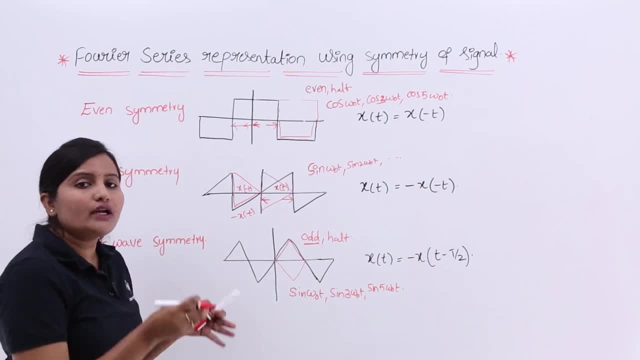 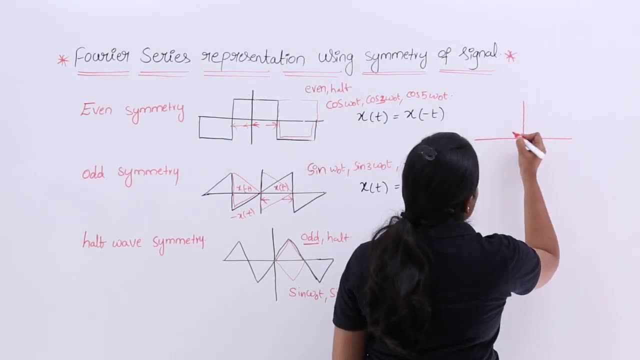 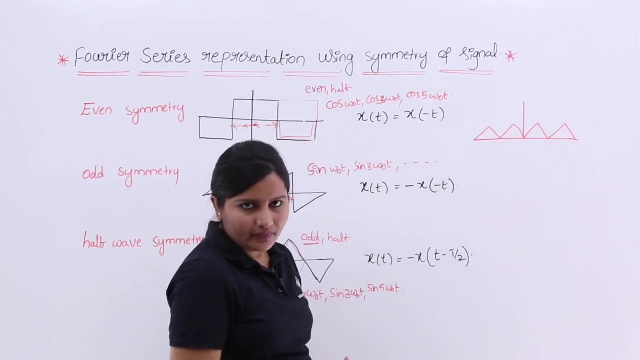 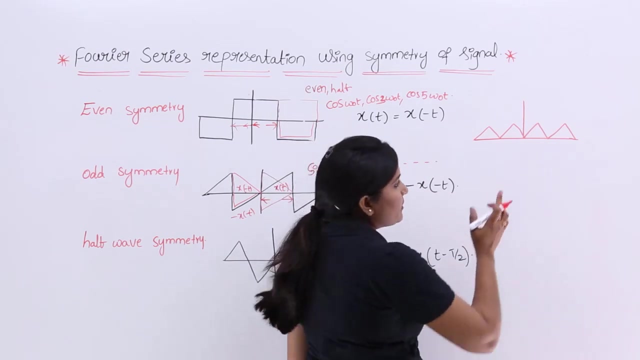 For example, you may get one doubt: what is the even, purely even symmetric signal which cannot satisfy half wave symmetry, For example? if you are having any signal like this, So you are having any signal like this. If you see this signal here, it is satisfying. just x of t is equivalent to x of minus t. that 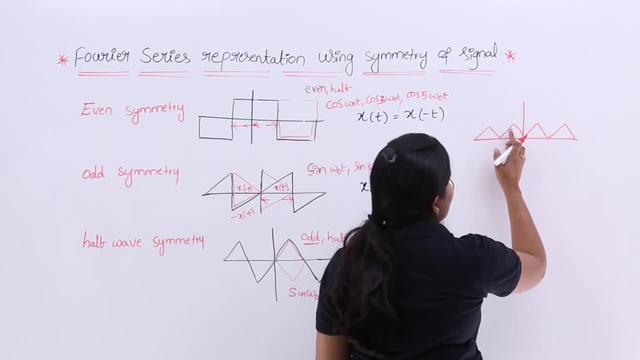 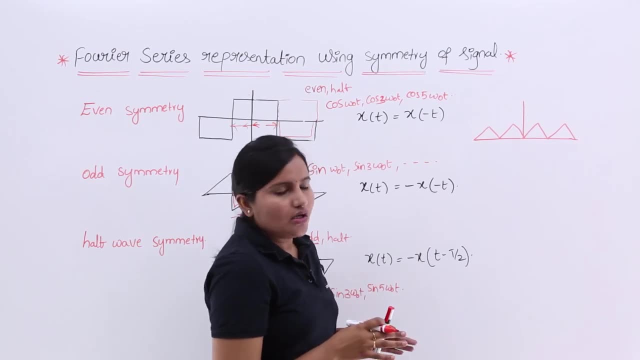 means. So here you are having, x of t is equivalent to x of minus t. the mirror image, whatever you are having there, that is exactly equal. So now you can say: this is even symmetric signal. whatever you are having in your positive side, same thing you are having on your negative side. 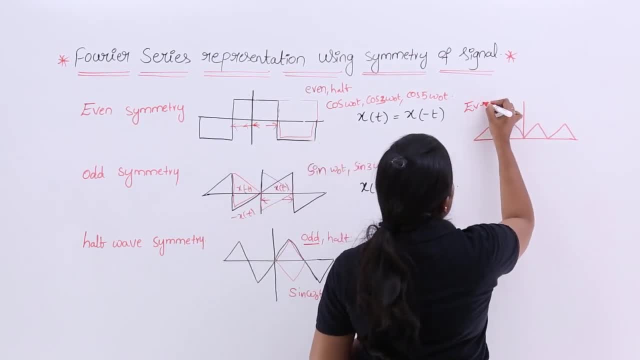 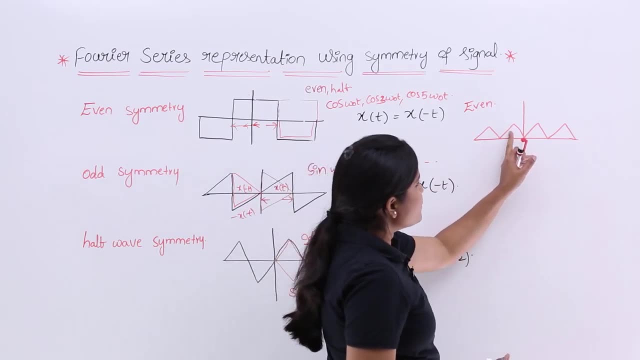 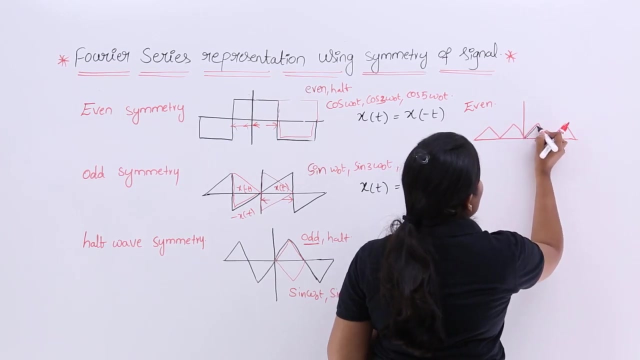 So you can say this is even symmetric signal. this is even symmetric signal If you want to check for any half wave symmetry, if you shifted and reverse. that means, for example, if you are considering this half and you want, you need to shift to check half wave symmetry and you need to revert that. 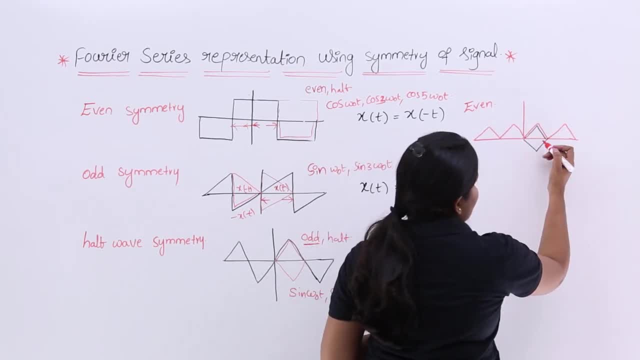 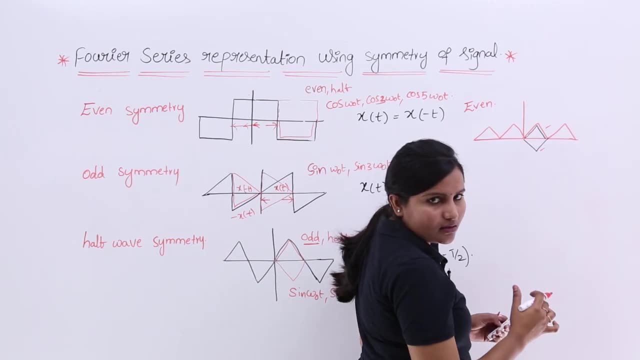 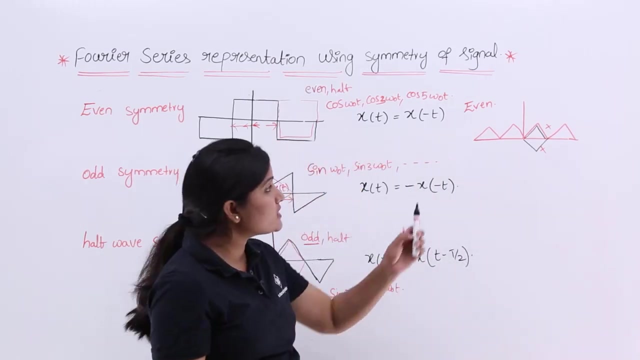 shifted signal. If you reverted that shifted signal, these two are not. the actual is in reading. So the shifted. So the shifted and reversed is in black color. So these two are not equal. So this is not satisfying half wave symmetry. this only satisfying. 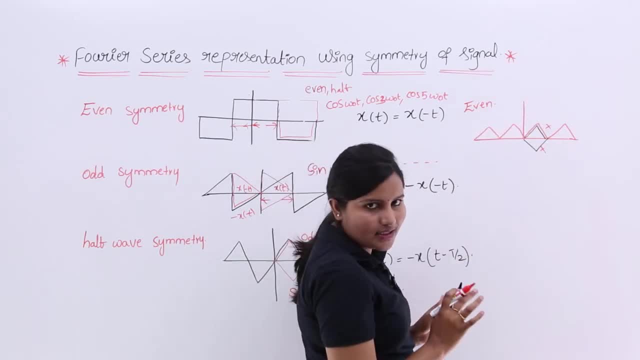 even symmetry. So for this signal, for this signal, if you want to represent Fourier series representation, then only cos terms, all cos terms are going to present. So all cos terms means cos 0, omega, naught, t, that means a naught, also will be presented. 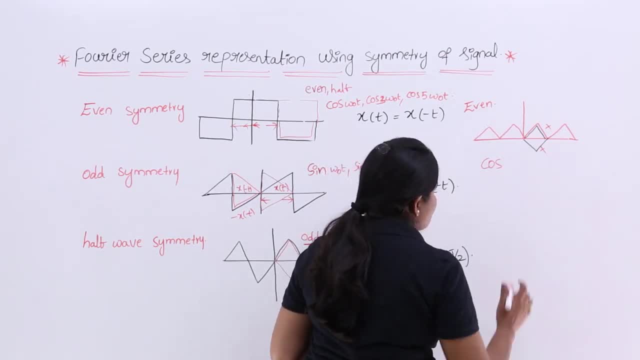 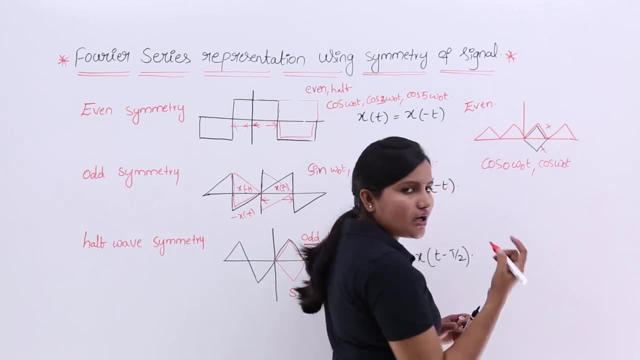 So here, So here. So that means A naught term is cos 0, omega, naught t, cos 2, cos, omega, naught t. all cos term means all odd harmonics, as well as even harmonics cos 2, omega, naught t, cos 3 omega. 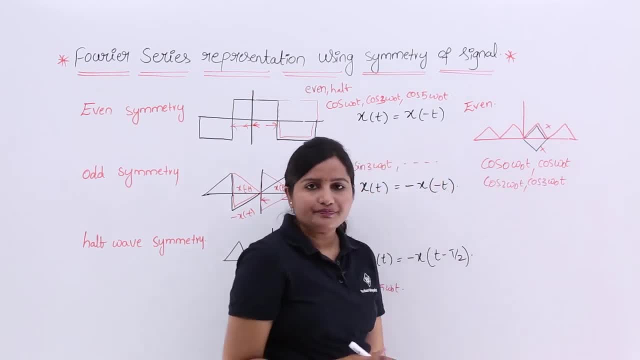 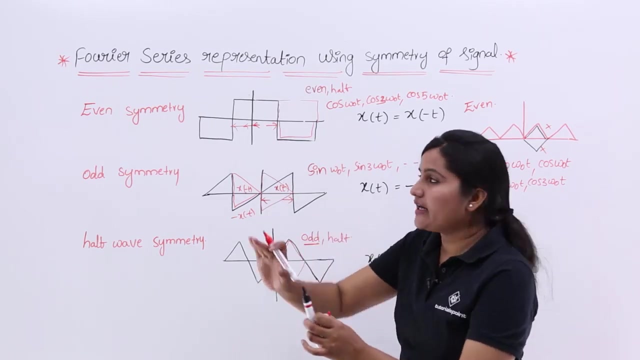 naught t all cos terms, including that constant is also going to present. So like this way, we need to check symmetry for the signal. So if you want to check even symmetry, whatever you are having in your right hand side, same thing you need to get in negative axis also. like this or like this, though these signals 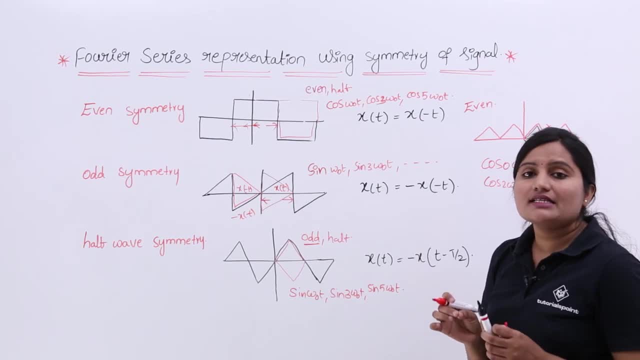 are said to be even symmetric signal When a signal is satisfying even symmetry. when you are representing Fourier series representation, it includes all the cos terms. So now odd symmetry coming to odd symmetry. if the signal is satisfying, x of t is equivalent to minus x. 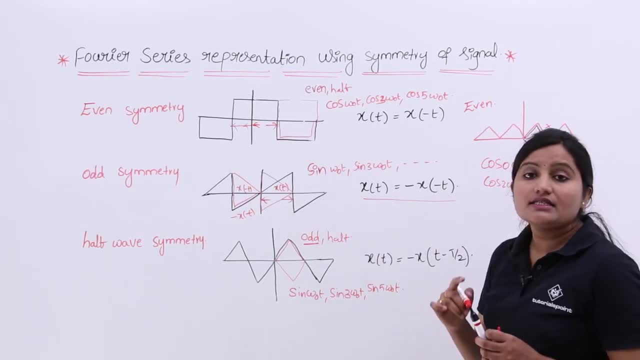 So x of minus t, then you can say that is odd symmetric signal. So this is purely odd symmetric signal. So coming to half wave symmetry. so to check half wave symmetry, the signal may be either even symmetric signal or odd symmetric signal. 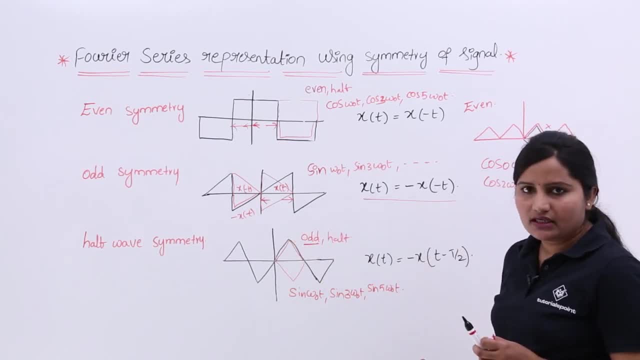 So here, for example, I consider odd symmetric signal to check half wave symmetry. if you consider this signal to satisfy half wave symmetry, this need to satisfy x of t is equivalent to minus x. So x of t minus t by 2, that means shift and revert the signal, here just image and 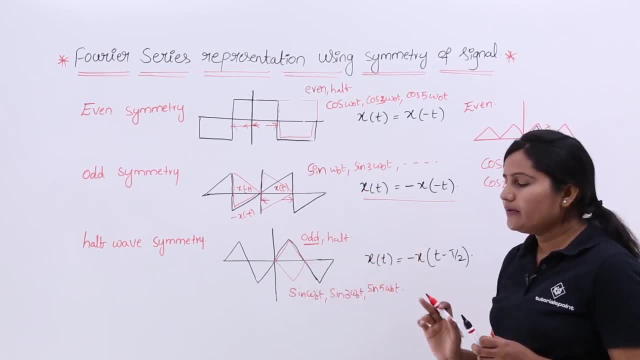 revert the signal, shift and revert the signal. So here here you are not getting you. here you are not getting any odd half wave symmetry here. here both odd and half wave symmetry are going to satisfy Whenever any even symmetric signal or odd symmetric signal is satisfying half wave symmetry. 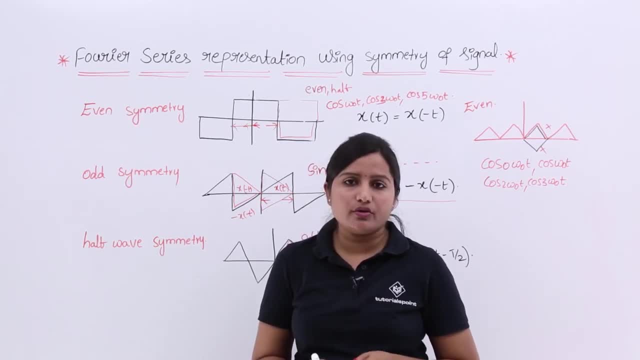 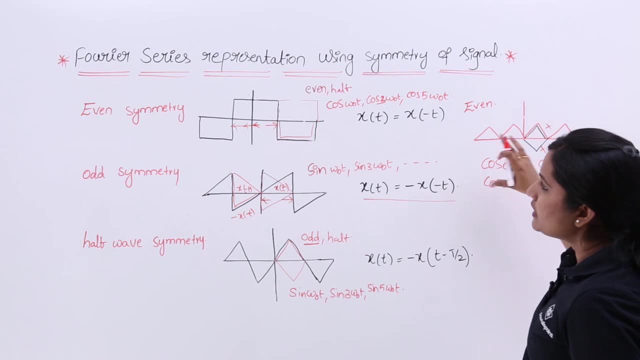 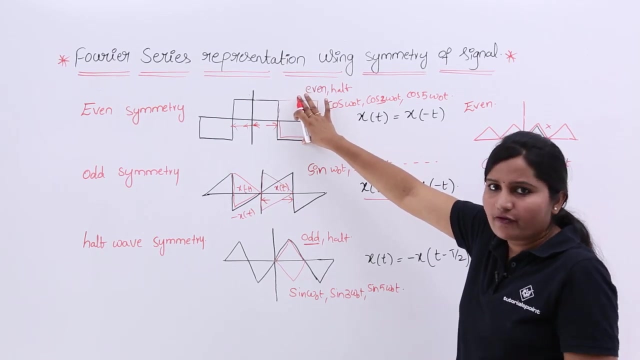 half wave symmetry, then only odd harmonics are going to be present. So, for example, this is purely even symmetric signal. all cos terms are going to present. this is not pure even symmetric signal. So this is even symmetric as well as half wave symmetric, only odd harmonics. 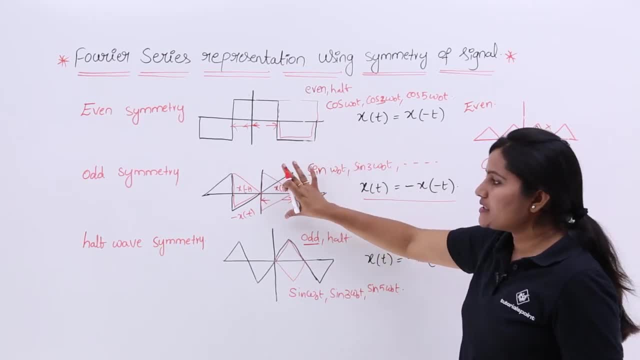 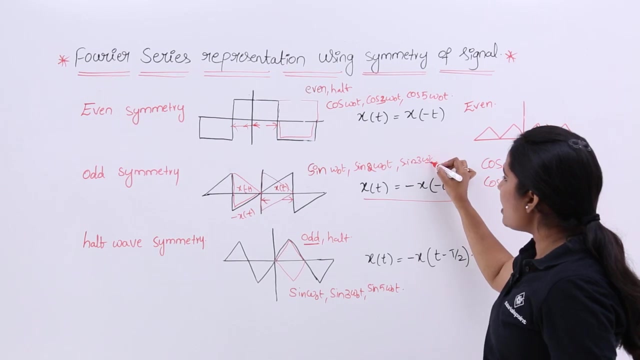 of cos are going to present. So now, this is purely odd symmetric signal, So all sign terms are going to present. So, if you consider this, all sign terms: sin, omega, naught t, sin 2, omega naught t, sin 3, omega, naught t. So all sign terms are going to present Now, 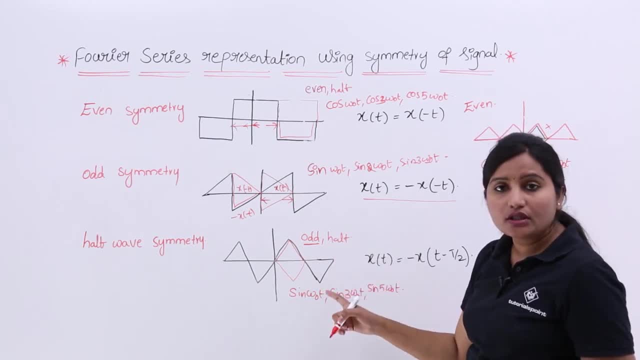 coming to this signal, this satisfying both odd and half wave symmetry. So now, so in odd odd symmetry also, that means in sign terms also, as it is satisfying half wave symmetry, we are going to consider Only odd harmonics of sin wave. sin signals why we are taking sin terms. because of it. 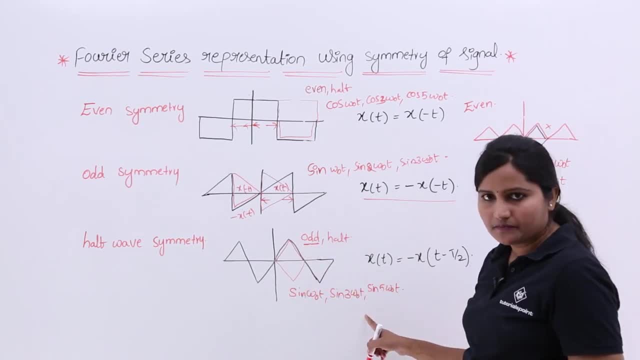 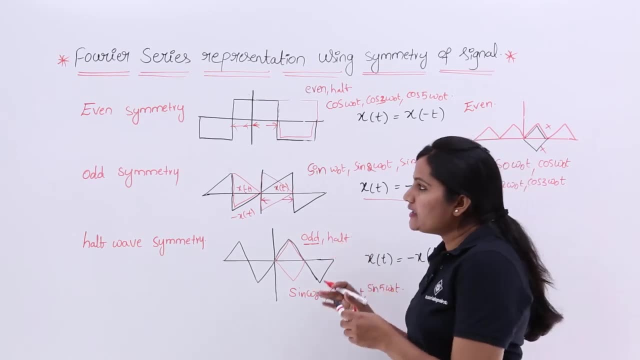 satisfying odd symmetry. that is why we are having only sin In that sin also why we are considering only odd harmonics, means it is satisfying half wave symmetry Like this way. we need to trace the answer how this topic is related to gate means. So in gate exam. 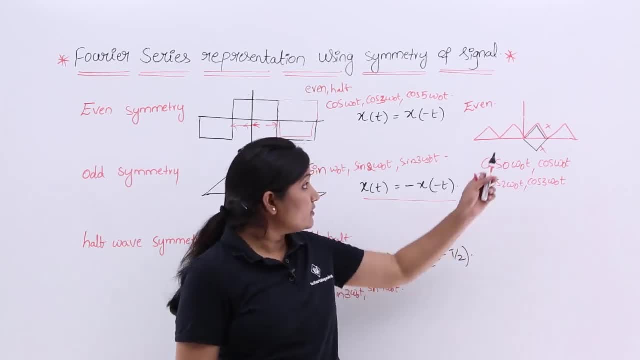 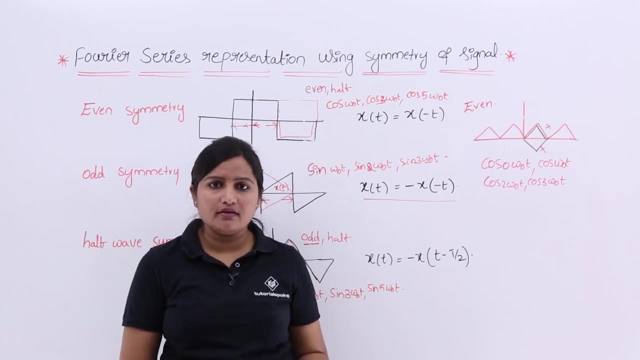 they will give any diagram. they will give this diagram, this diagram, this one or this one. They will ask: what is the Fourier series representation of that signal? They will give options In that, options without doing Fourier series representation generally. how we will do Fourier series representation? first of all we need to take the definition of the 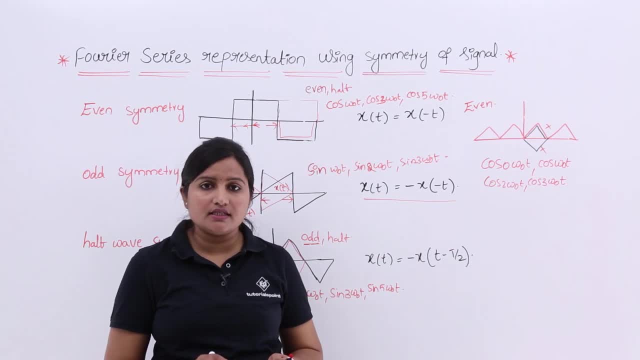 signal and we need to substitute in trigonometric Fourier series and we need to consider the values of a, n, b, n and a naught. We need to substitute a naught, b, n and a, n values again into that general equation. Then only you are going to get your final result of representation Doing that process. 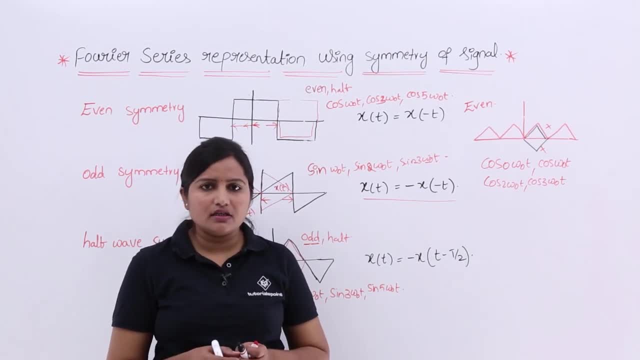 will nearly take half an hour to trace the answer without any confusion. you need to apply symmetry for that problem. If you apply symmetry, if that is purely even symmetry, whatever the option is having all cost term that you need to select. If that is satisfying, when is even? 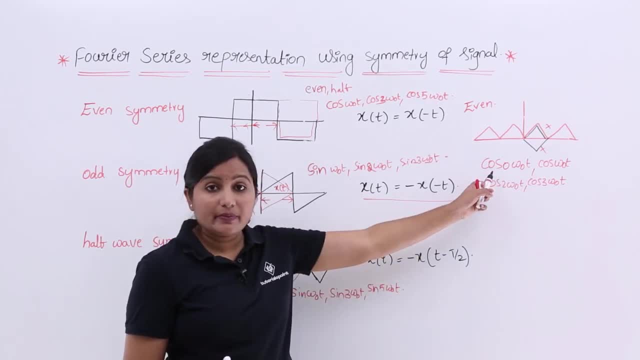 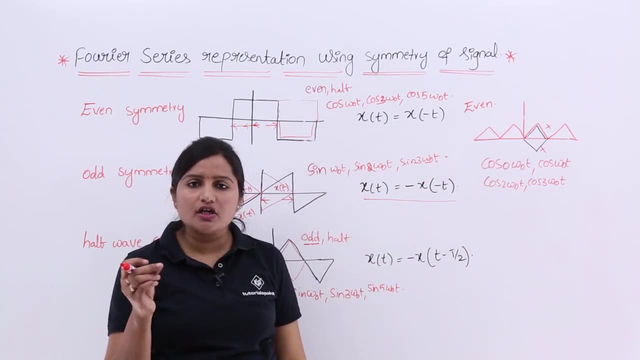 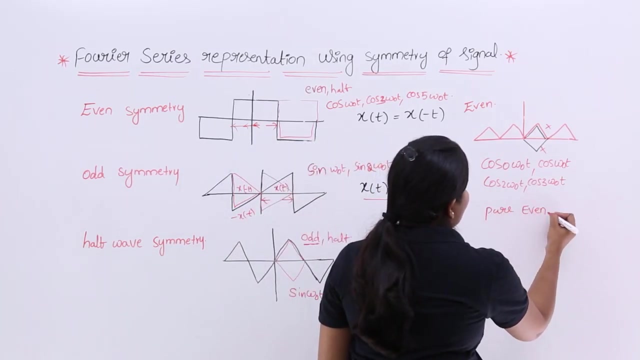 symmetric, then only a n will be present. Why? because so 0 omega naught is also considered as even harmonics, So 0 omega naught is means a n term when a pure, even symmetric signal is there, pure, even symmetric signal, So that constant term will be there, constant term. 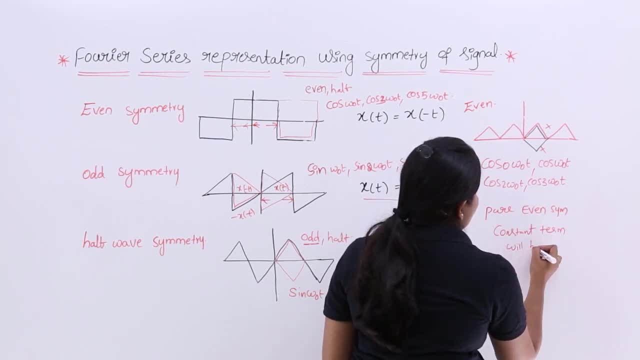 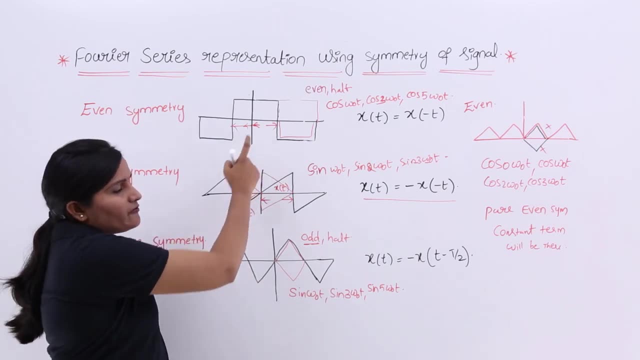 will be there, For example, if you are having this type of signal, if you are having this type of signal, this is also even symmetric signal. but here there is no coefficient, there is no constant. Why? because here this is satisfying both, even symmetry as well as half wave symmetry. then